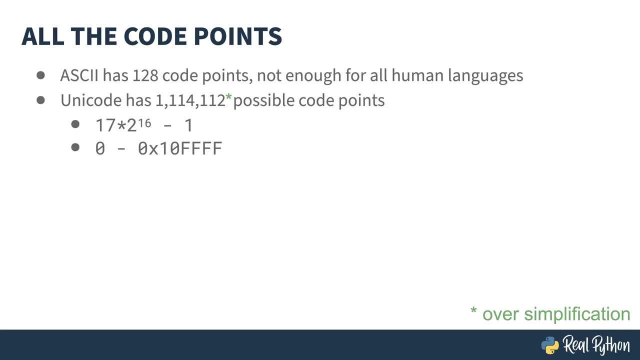 so the full range isn't actually available, but the number's close enough between friends. The first 128 code points in Unicode are ASCII, making it backwardly compatible. Unicode itself is not an encoding. Unicode really only specifies the map of the code points. Unicode itself is not an encoding. 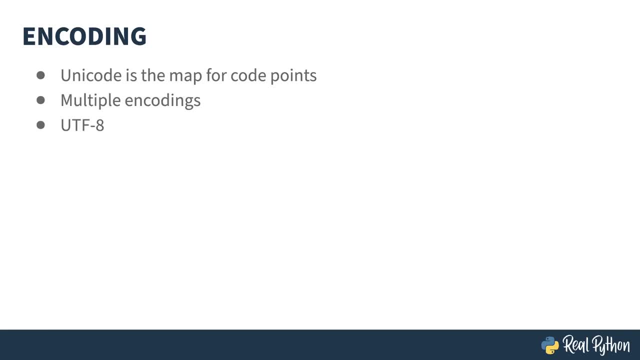 It's a map for the code points. UTF-8,, the basis for Python, is the most common and popular of the encodings. There's also UTF-16,, 32, and actually several others. Python 3 has two representations of data: strings and bytes. 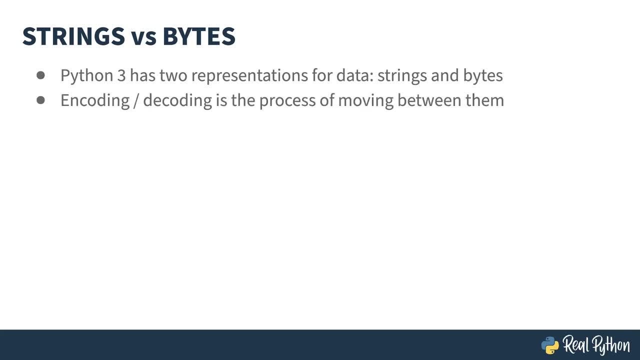 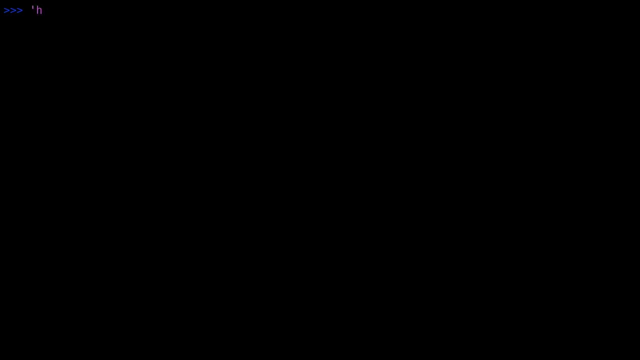 Bytes are straight, binary strings are text. The concept of encoding and decoding in Python is the process of moving between these two representations. Let's start off with a sample encoding. Here's good old hello encoded into UTF-8, and you get back the binary representation hello. 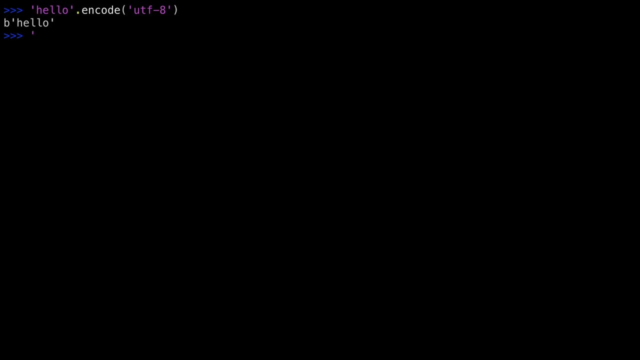 For ASCII. it's pretty simple. There's not much change. Let's look at something a little more complicated: Café encoded CAF: still ASCII, But E- l'accent aigu- is not inside the ASCII table. UTF-8 represents this letter using C3A9 hex. 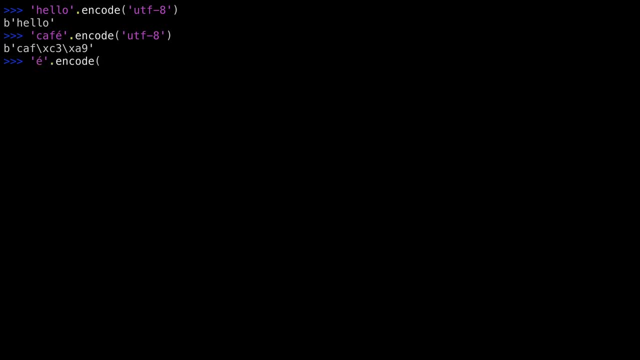 To highlight that. let's look at it in a different way. Let's look at it on its own. Same result: Charlie 3,, alpha 9.. The UTF-8 encoding is actually variable length. Anything in the ASCII table is represented by a single byte. 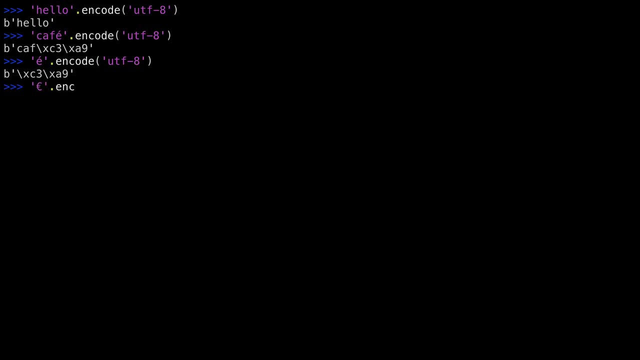 The E in CAFé is two bytes. The euro symbol is actually three bytes. encoded. UTF-8 can go all the way up to four bytes encoded. The decode method does this backwards. So by starting with CAFé, hex C3,, hex A9, decode and you get back to the original string. 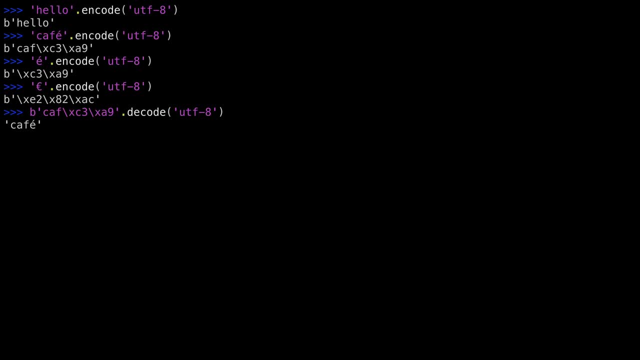 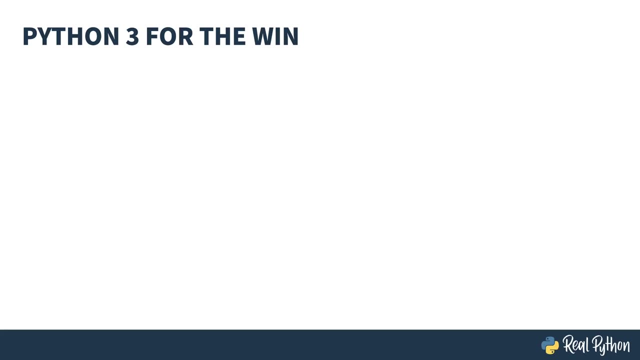 Notice that you're feeding this decode method a binary representation and it's returning the string result, the opposite of the encode method. Later versions of Python 2 did support Unicode, but they did so by adding a layer on top of ASCII, and it caused all sorts of complications.